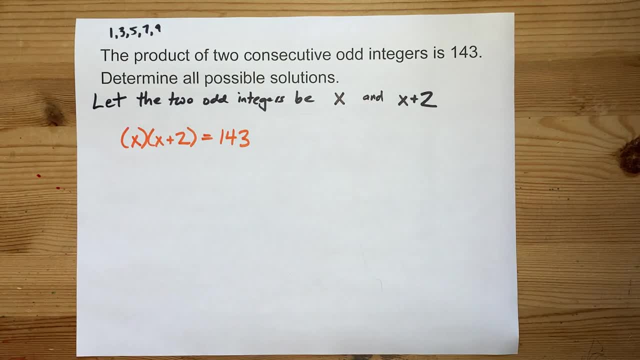 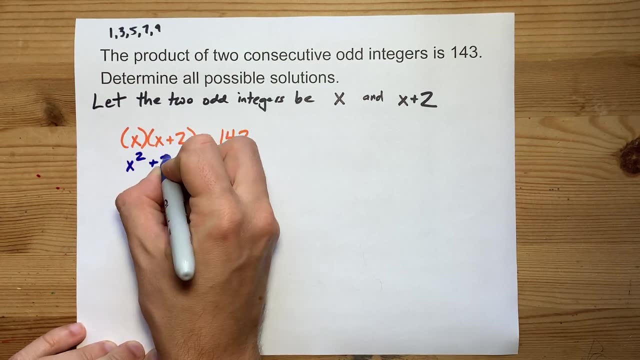 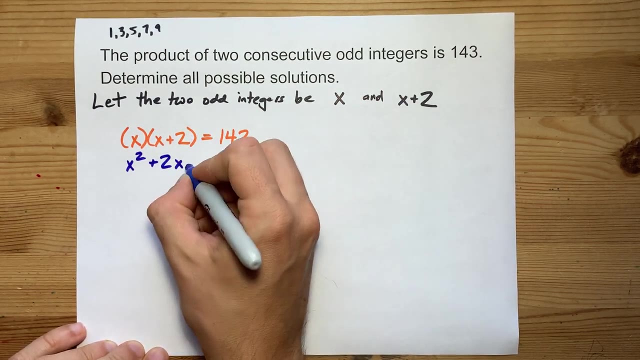 are always easier to solve when one side equals zero. So multiply, multiply. I'm going to distribute the x through the brackets. I get x squared plus 2x there, And just because I'm flexing, I'm going to move the 143 to the other side at the same time. 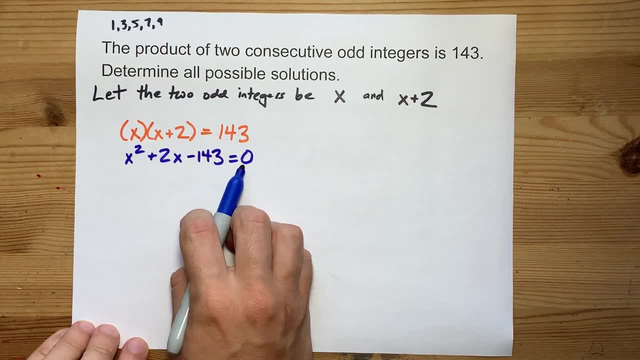 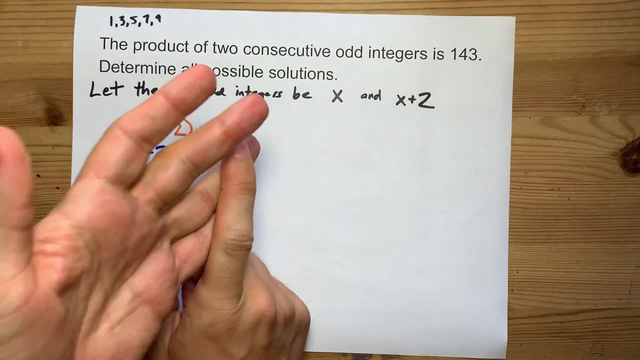 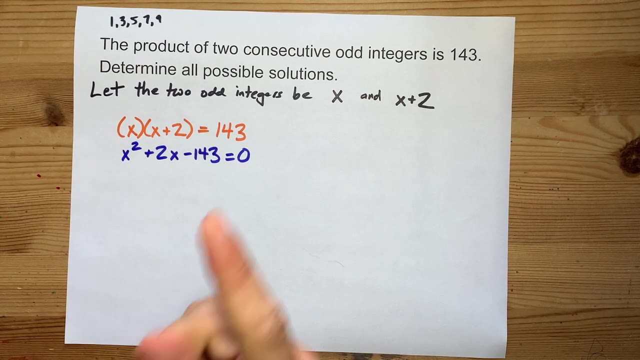 There we go. I got x squared plus 2x minus 143 is zero. Now you can solve this by either factoring or completing the square- if you know what that is- or quadratic formula. I happen to know that this one factors. We're looking for two numbers that multiply something times something else. 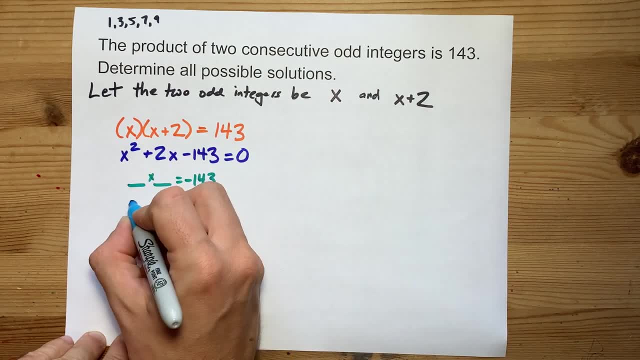 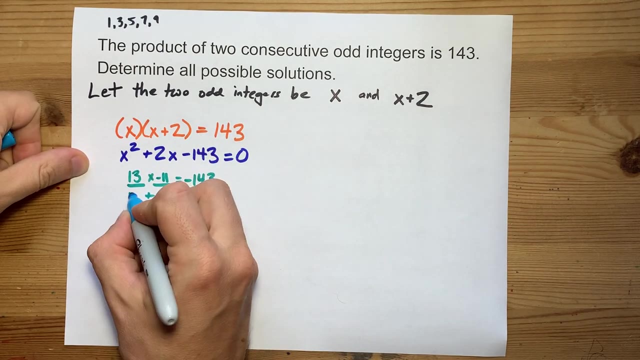 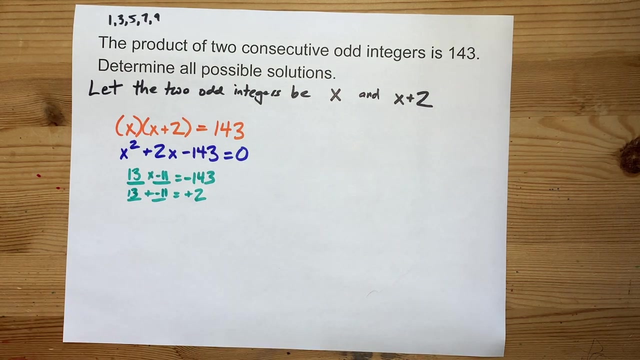 gives negative 143. And those same two numbers will add to give us 143.. And so we're going to positive 2.. Now I know what those numbers are. It's positive 13 and negative 11.. Positive 13 plus negative 11 is 13 minus 11,, which is positive 2.. It all works out. Let me just 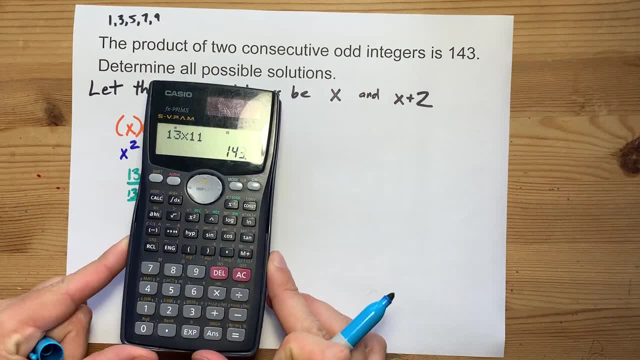 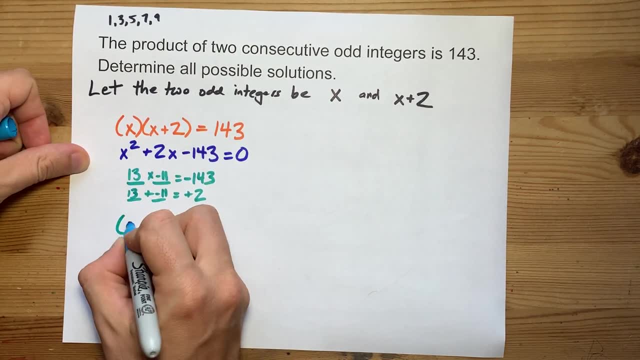 verify that on my calculator, 13 times 11 is 143.. Beautiful. Once you've found your magic numbers, you can plug them straight in to the factored form. If you know, the numbers are positive 13 and minus 11, and there's no coefficient on x squared. 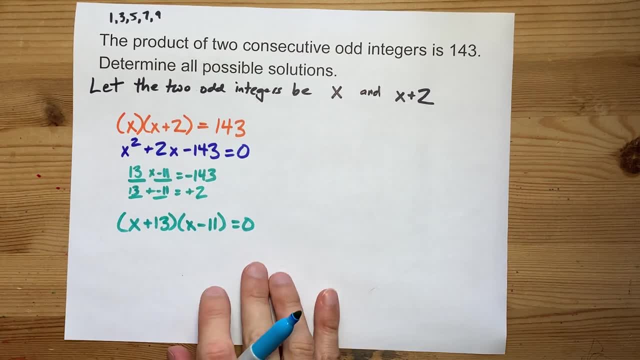 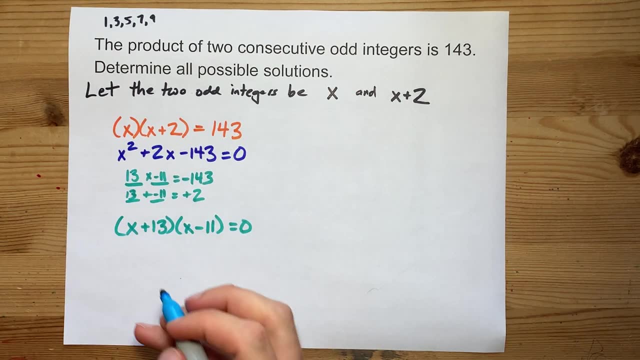 there's a shortcut to get to this version of the factored form. Now we have this factor. times this factor equals 0. That means like if two numbers multiply to make 0, then either x plus 13 equals 0, or x plus 13 equals 0. So if you know the numbers, you can plug them straight in to the. 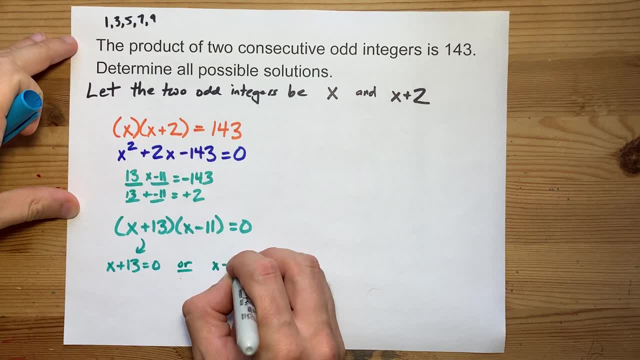 factored form. Now we have this factor. times this factor equals 0. That means like if two numbers multiply to make 0, then either x plus 13 equals 0, or x minus 11 equals 0. It's your job to solve for x in both of these cases. Here something plus 13 is 0. You can move the 13 to the other side- 0 minus 13.. So I get negative 13 out of that. Here I could move the minus 11 to the other side. It becomes plus 11.. X is 11.. Oh, okay.